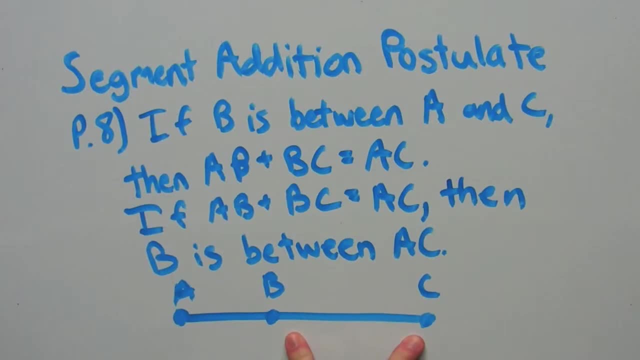 then the measure of this segment plus the measure of the BC segment equals the measure of the entire segment. And that is what this postulate is saying up here. If B is between A and C, then AB plus BC equals AC. Or if AB plus BC already equals AC, then B has got to be between A and C. 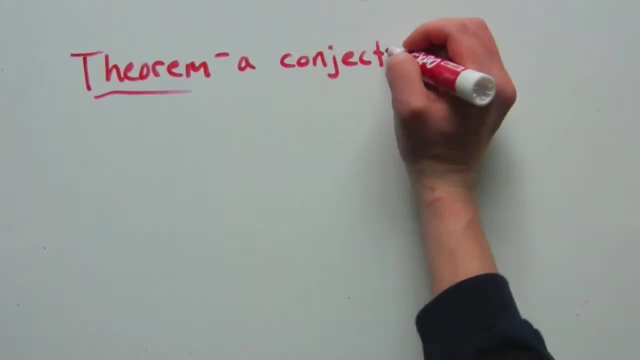 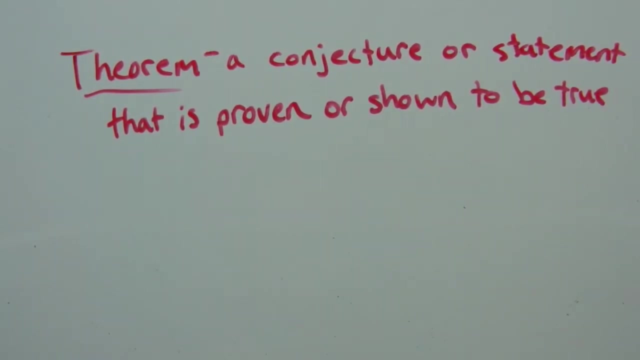 So in this case we are going to have to prove that the conjecture is true. So a theorem is a conjecture or a statement that is proven or shown to be true, But how do you prove or show that that conjecture is true? 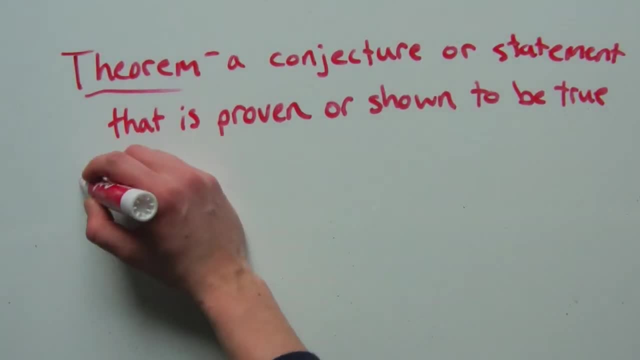 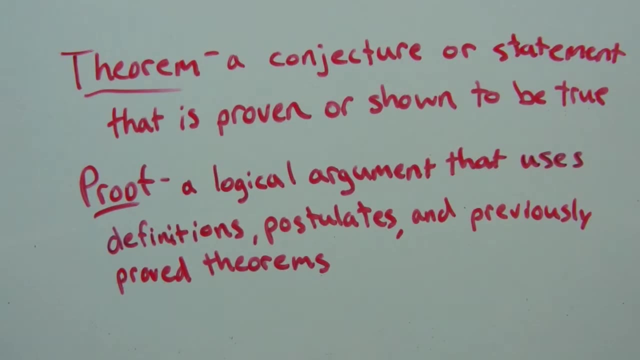 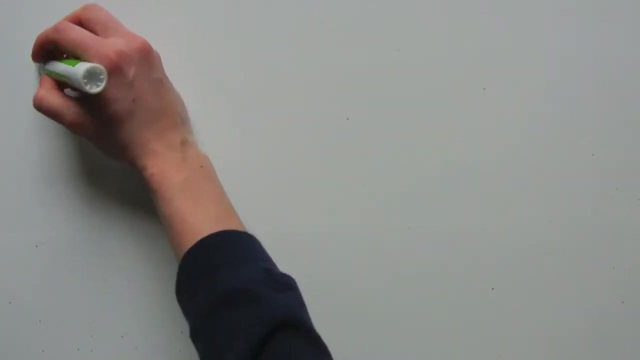 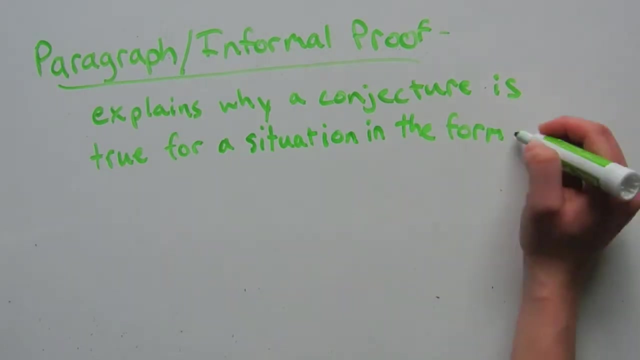 That's where proof comes into play. Okay, So proof Is a logical argument that uses definitions, postulates and previously proved theorems. So now we're going to talk about one form of a proof. So a paragraph or informal proof explains why a conjecture is true. 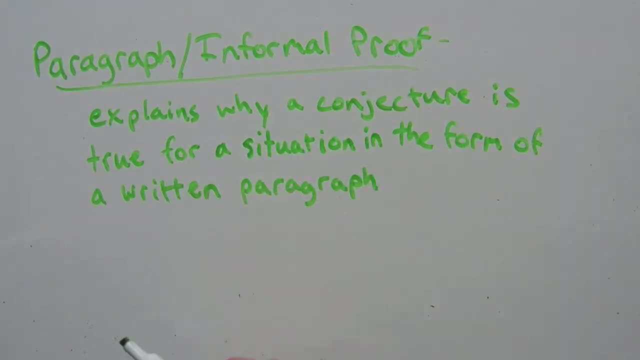 for a certain situation or a given situation in the form of a conjecture. So a conjecture is a conjecture that is proven or shown to be true. It's proven or shown to be true like we'veですね. that's a form of a written paragraph. 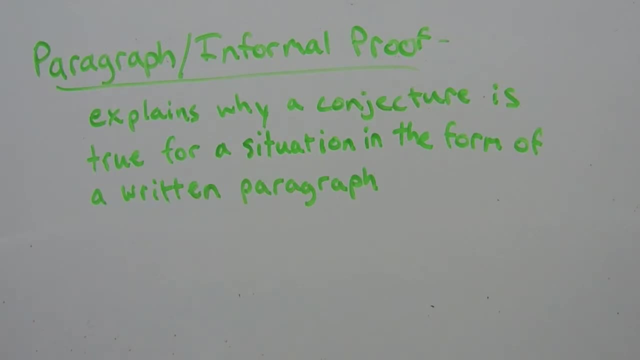 but how do we even start to make that proof? Well, here's five simple tips to help you formulate a proof. Step one: most books will say: state the theorem or conjecture that is to be proven, and most times that's given to you what you need to prove. 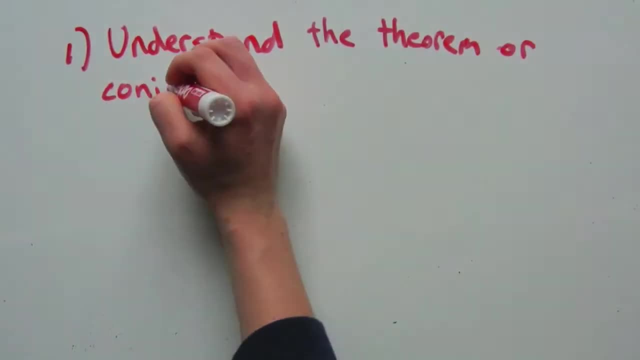 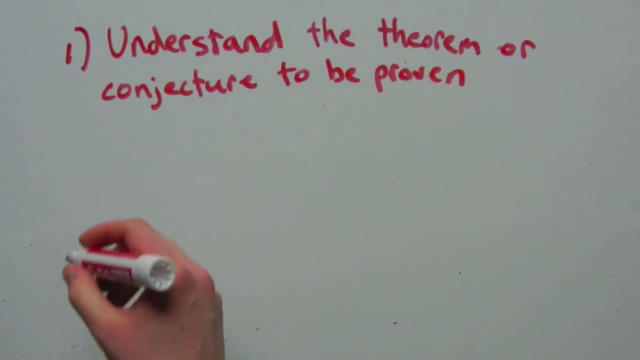 but I think, more so than stating it, you need to understand that theorem or conjecture. Okay, so step one. So understanding the theorem or conjecture to be proven is step one. Step two: you're going to want to list the given information. 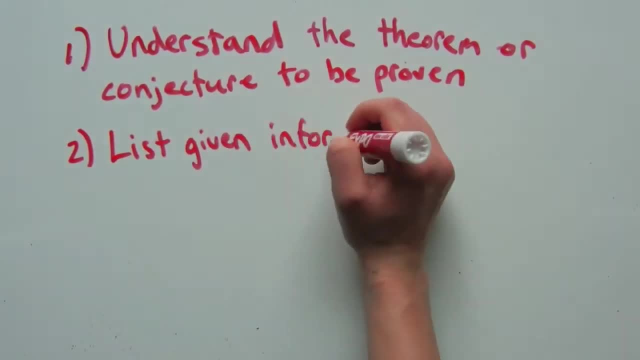 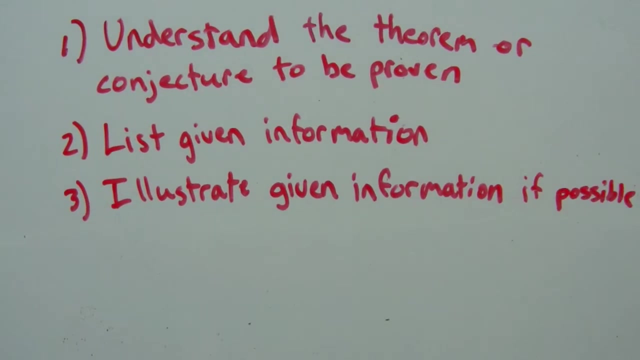 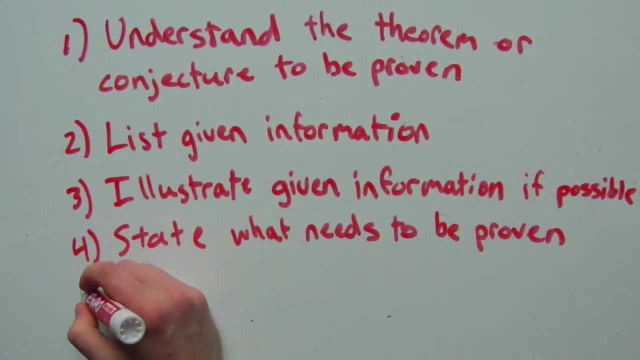 So list what the problem gives you. The next step, step three, is, if possible, we're going to want to illustrate that given information in a picture or diagram. So illustrate that given information, if possible. Our fourth step is to state what needs to be proven. 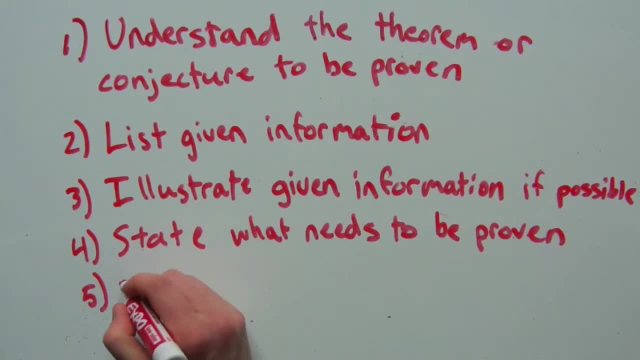 And finally, number five: develop the steps. So understand the theorem or conjecture to be proven, To list the given information, Illustrate the given information, State what needs to be proven And then develop those steps. And developing the steps really vary depending on what you're trying to prove and your favorite. 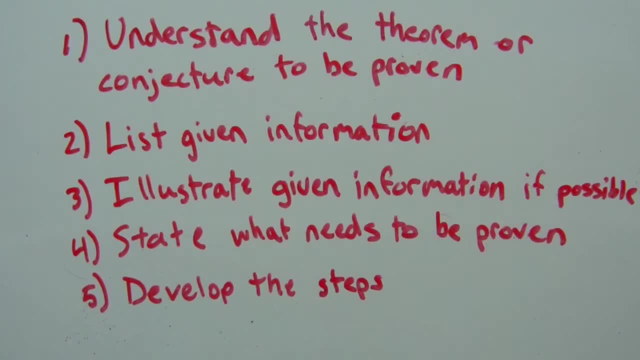 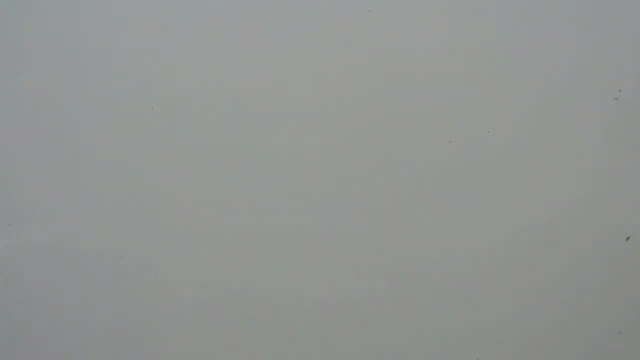 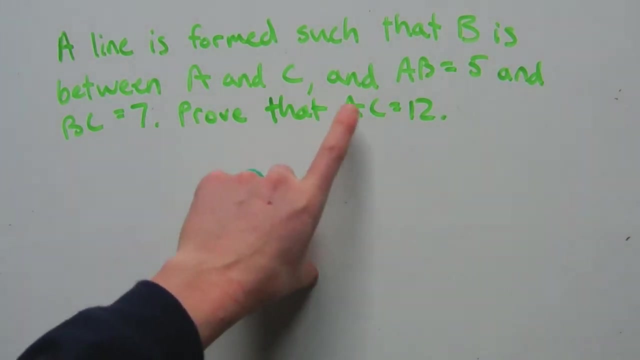 method for developing those steps. So now let's utilize these steps and do our first proof. Here's our problem. A line is formed such that b is between a and c and ab equals five and bc equals seven. Prove that ac equals twelve. 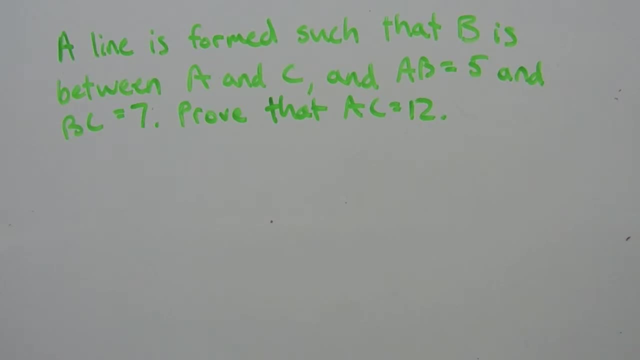 So the first thing we're going to do is understand the theorem or conjecture that is to be proven. So what we need to prove is that ac is equal to twelve, And that's easy enough to understand, because twelve is the measurement of a segment a. 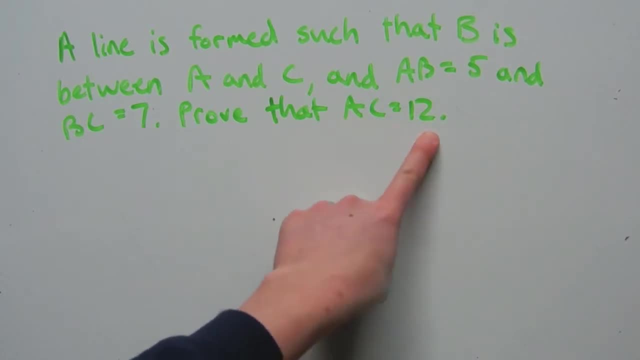 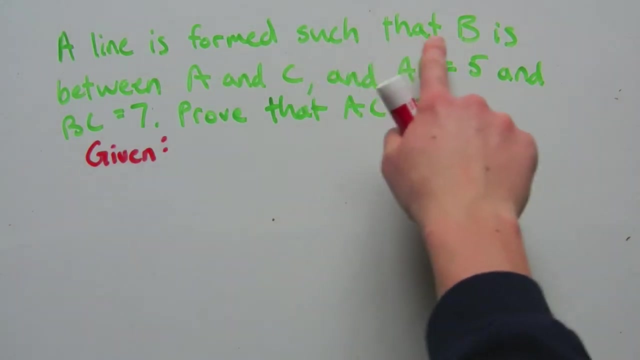 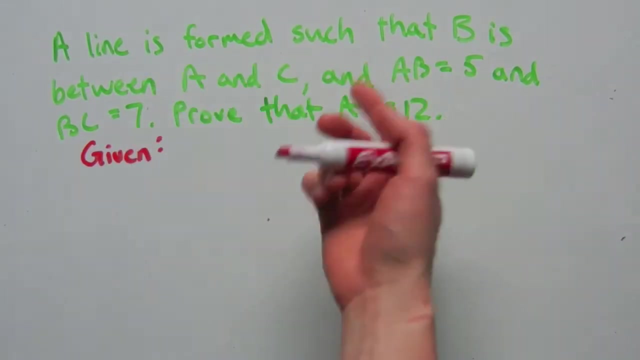 c. So we need to prove that that measure is twelve. Now our next step. number two list the given. So given we're given that b is between a and c Because it says that a line was formed such that b was between a and c. 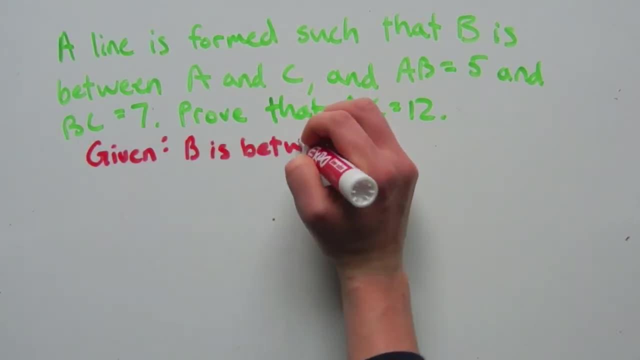 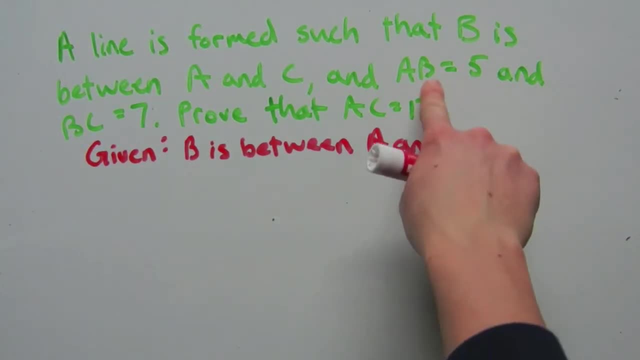 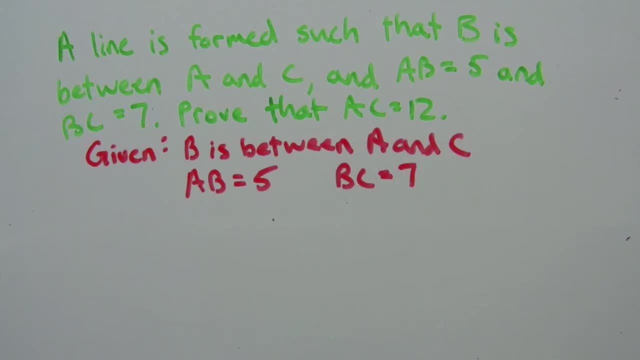 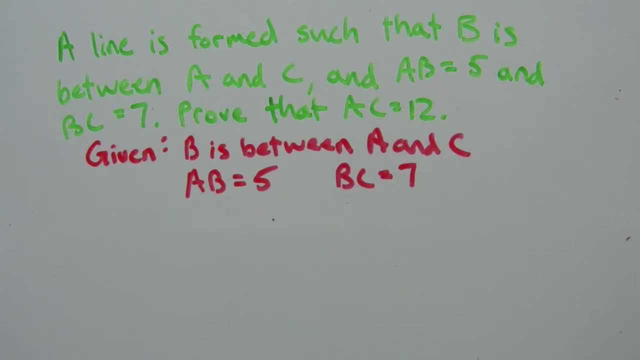 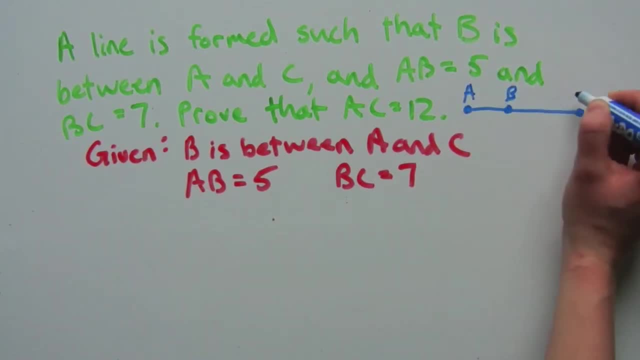 We have a, b is between them, and then c, and we have that ab is equal to 5, and bc equals 7.. So that's just a quick sketch of the given information. Now we need to state what needs to be proven, or true? 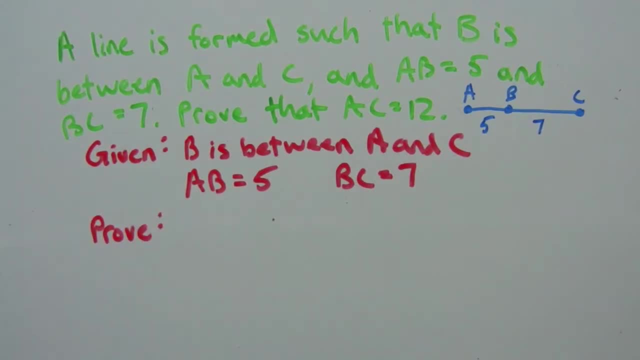 So prove ac equals 12.. So we're proving that ac equals 12.. Now we're going to develop the steps. How do you think we're going to go from this given information to the statement or conjecture that needs to be proved? 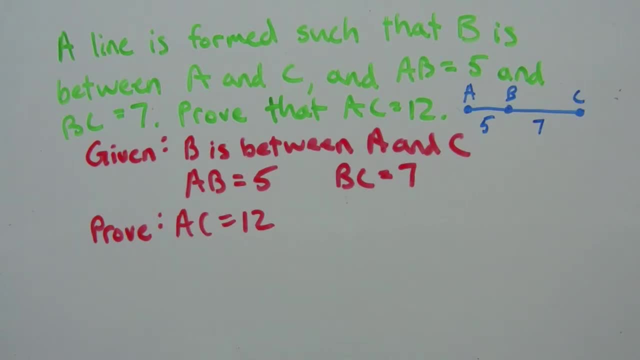 In the very beginning of this video we went over a postulate- It was the segment addition postulate- And that's going to be used to prove this statement. We're doing an informal proof, so we're going to write in paragraph form our proof. 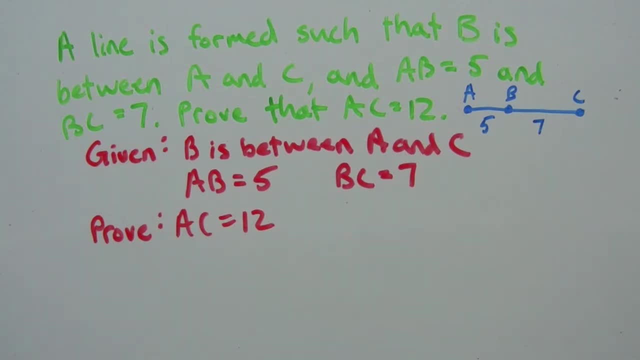 And that's where we're going to write all the steps that we do to prove that. So, number five, developing the steps. Okay, So first we have, since that b, our given information is between a and c from p8, which 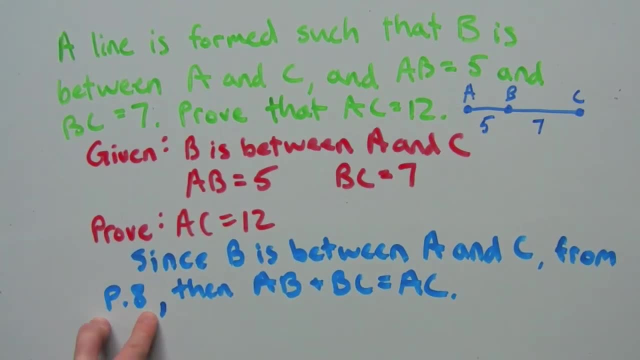 was the segment addition postulate. I just wrote p8 here so I didn't have to write out all the words. then we have that ab plus bc equals ac And the postulate was that if b is between a and c, then ab plus bc equals ac. 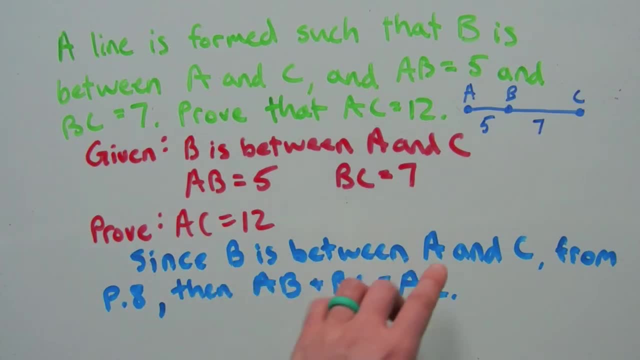 And a postulate is true, So it is safe to assume that, since b is between a and c, in this problem ab plus bc is equal to ac. And remember, what we're trying to prove is that ac is equal to 12. And we're given that ab and bc are both a certain measure.